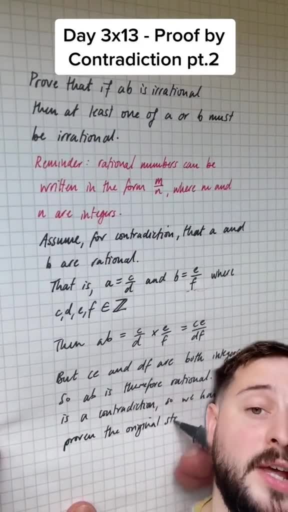 statement is true, meaning that if AB is irrational, then at least one of A or B must also be irrational.